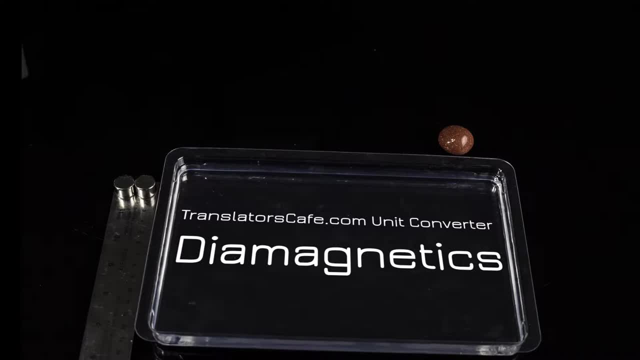 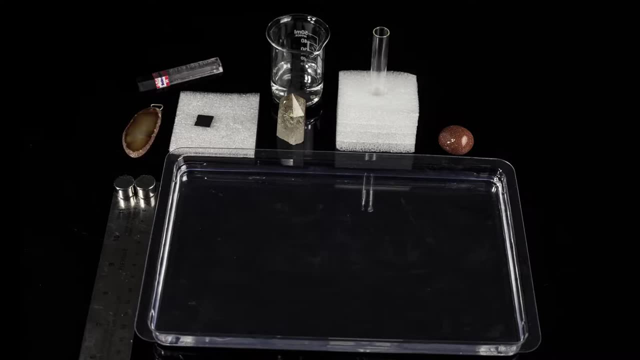 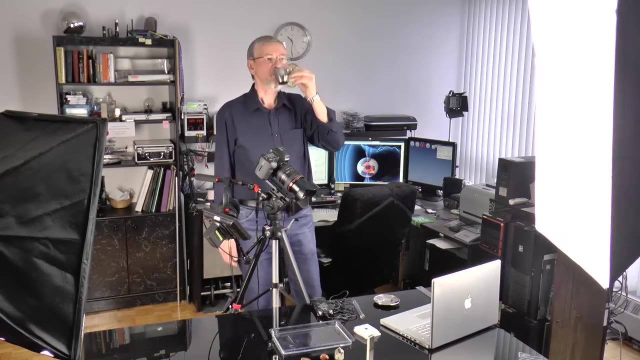 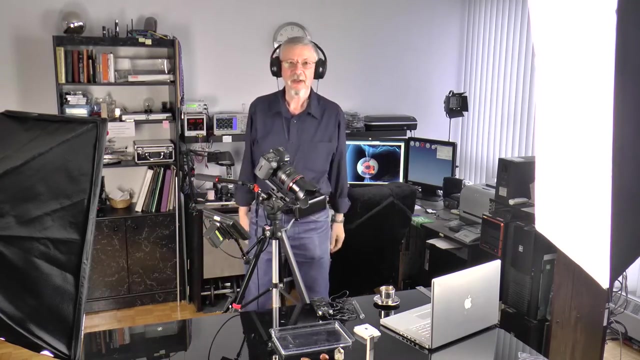 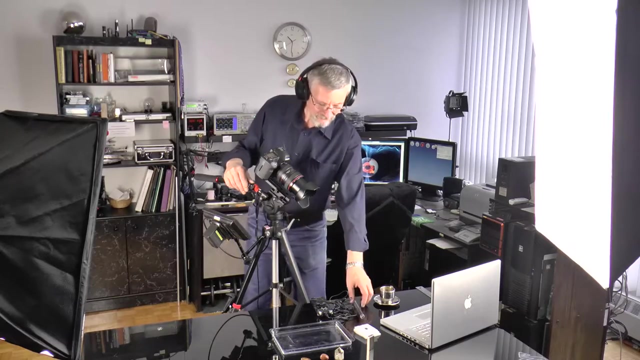 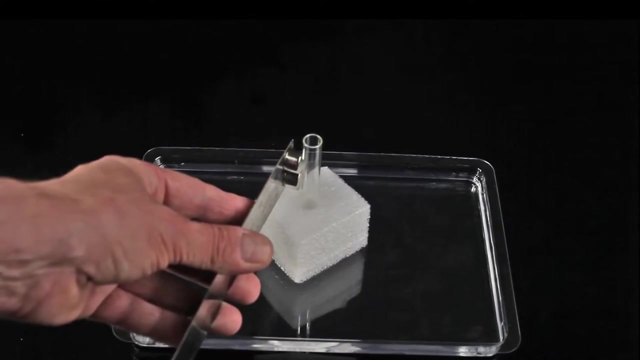 Hello and welcome to the TranslatorsCafecom channel. I will demonstrate magnetic properties of glass, water, graphite and some other materials. To observe very small forces, we will use some foam floating in water In the strong magnetic field of a neodymium magnet. diamagnetic materials such as glass agate or quartz. 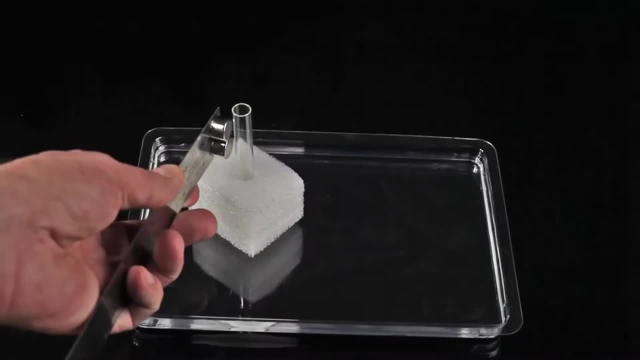 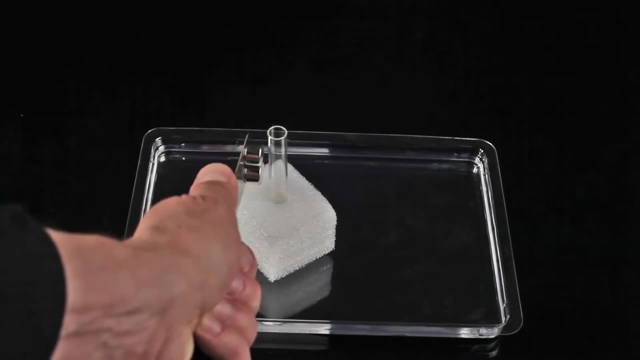 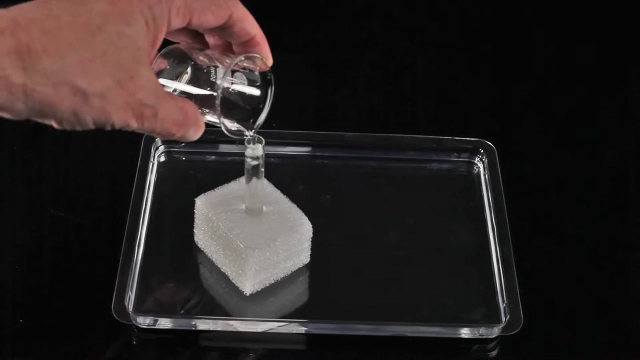 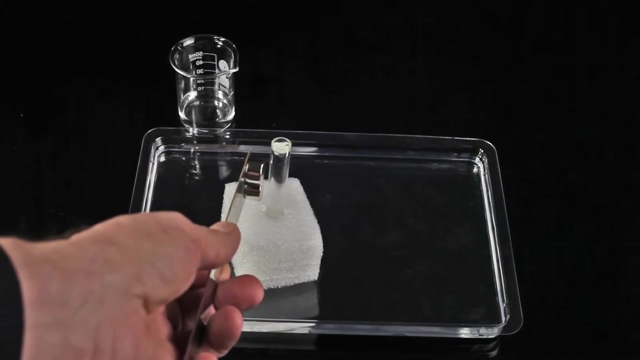 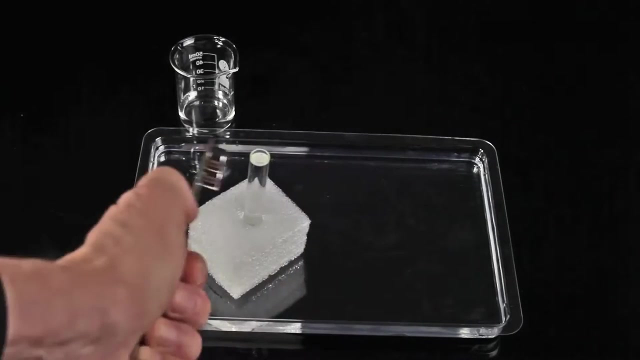 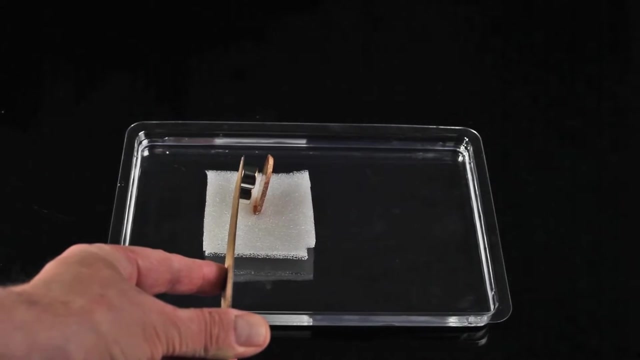 create an induced magnetic field in the direction opposite to the external magnetic field. As a result, they are repelled by the applied magnetic field. We can see that water has stronger diamagnetic properties than glass. Agate mainly consists of silicon dioxide, commonly called silica. 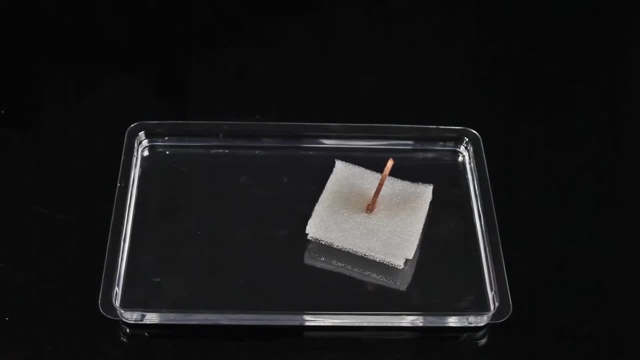 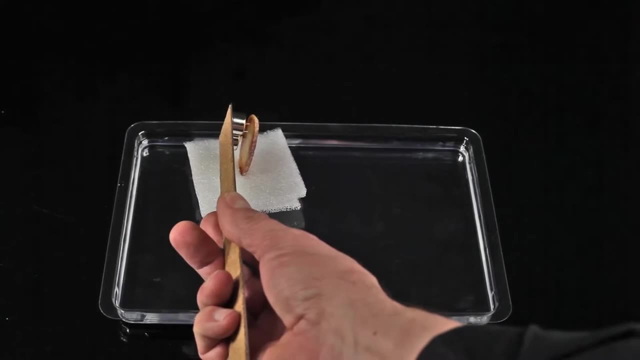 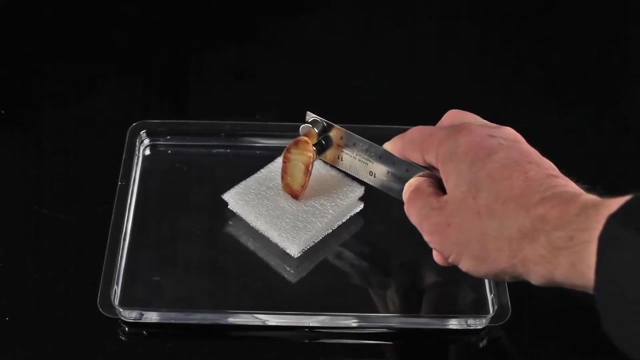 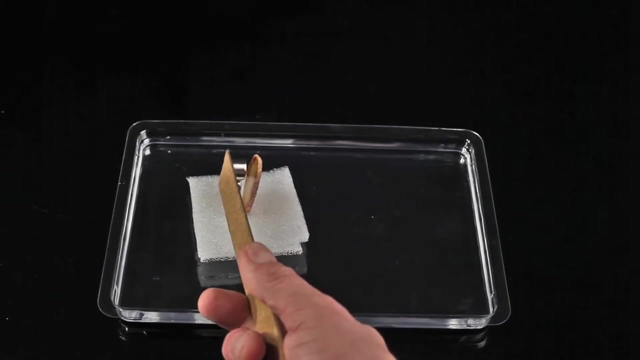 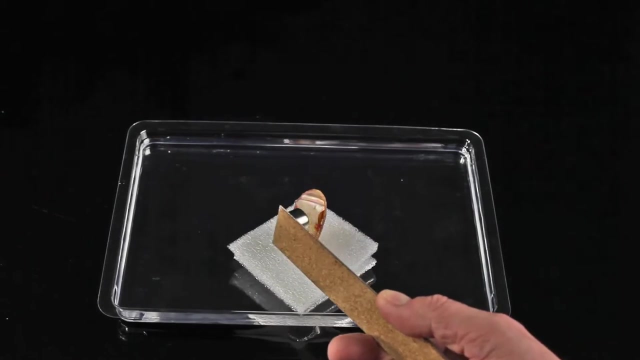 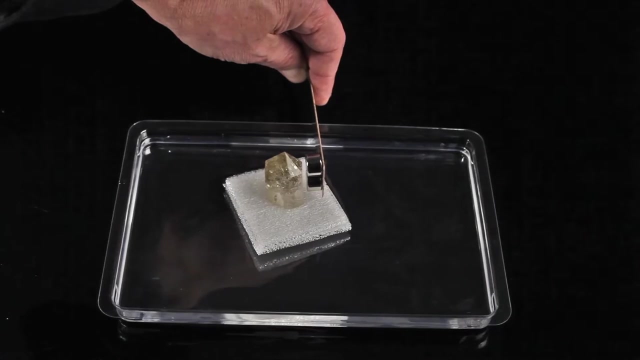 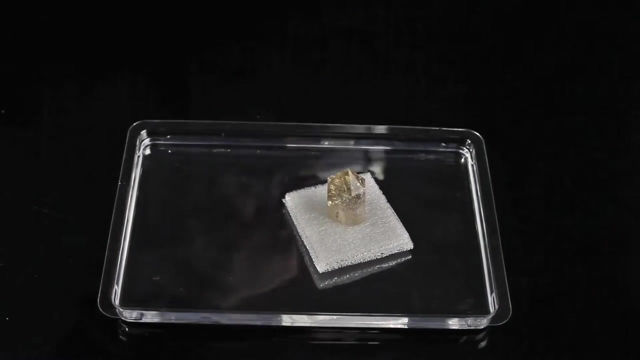 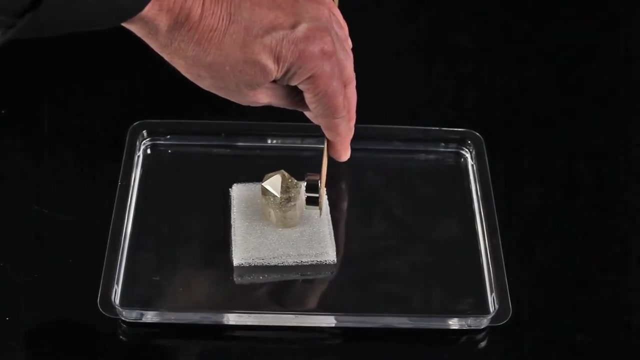 Glass is also based on silica because it is made of sand, So we can expect that agate is also paramagnetic, and this experiment confirms it. The same is true for quartz. Quartz is another mineral made of silicon dioxide and, as you can observe, it is also repelled by a magnetic field. 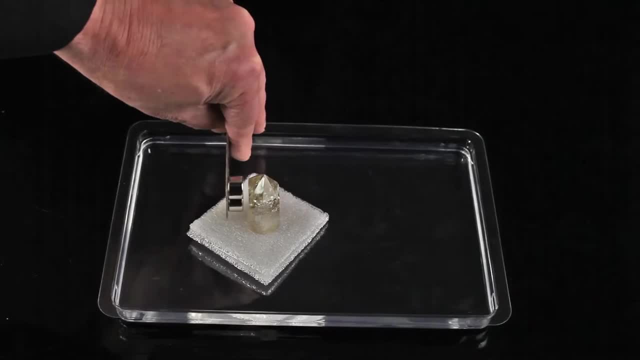 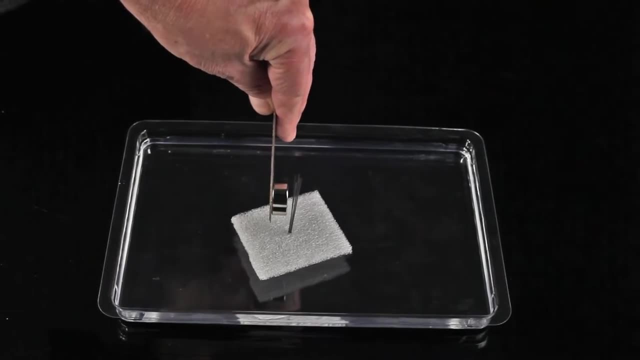 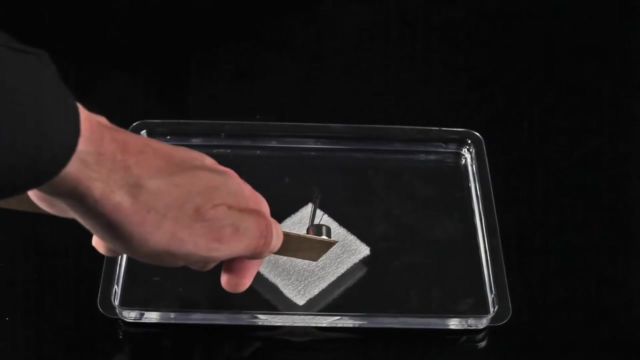 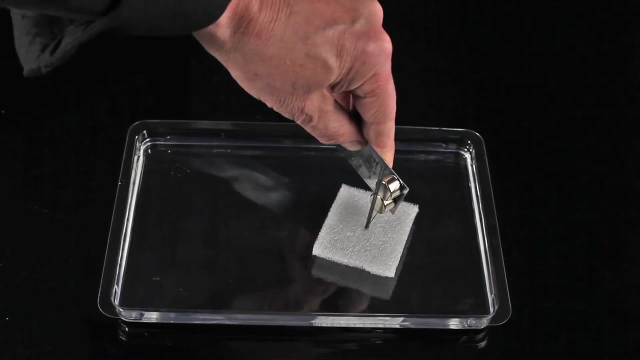 Therefore, it is salt-solubleラ. These pencil lids are made of graphite mixed with clay and, as you can see, they are repelled by a magnet. P不會 раст học. ca. 05.5 emission. 06.2 emission.